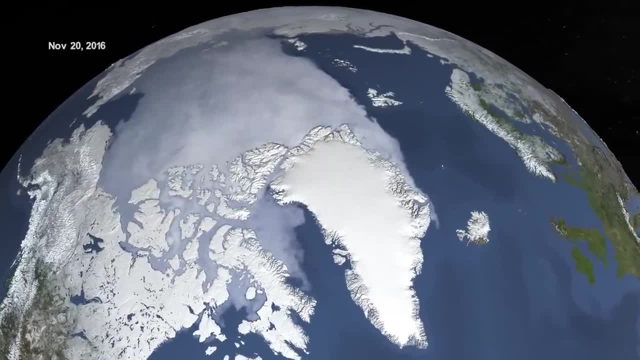 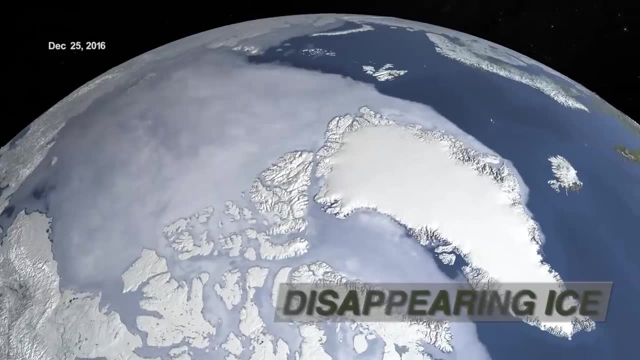 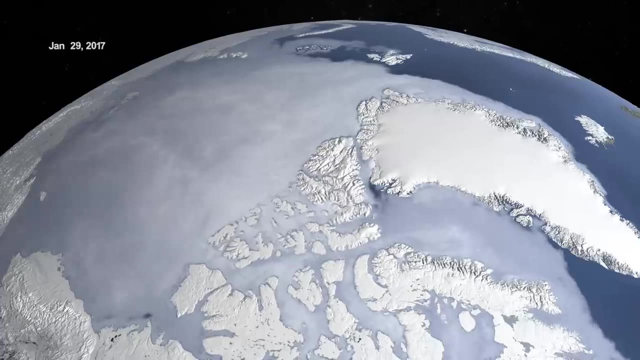 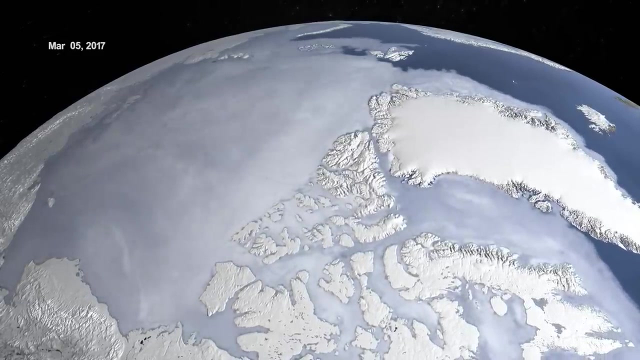 In 1978, satellites began continuously observing the polar regions and the dynamic beauty of the Arctic sea ice was revealed. What we expect to be a solid mass of ice is actually in constant motion As researchers continue to seek a deeper understanding of this region. 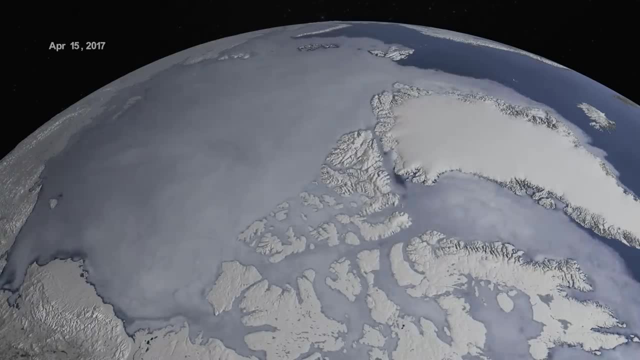 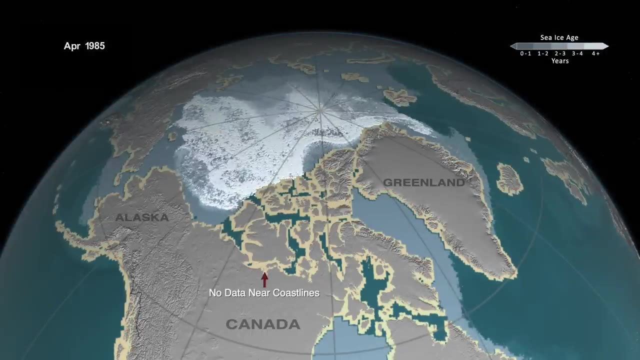 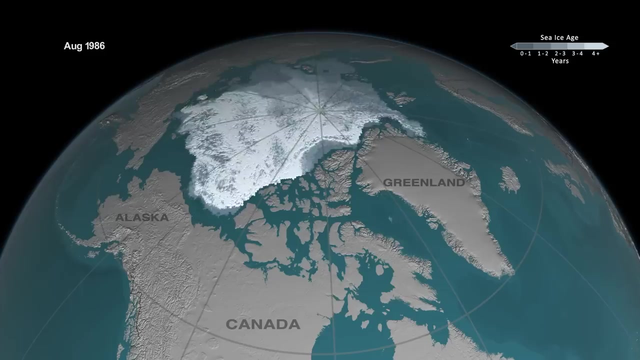 new information about how sea ice changes is coming to light. In this animation we're taking Arctic sea ice into the third dimension. Here we're looking at the ice age, which is an indicator of thickness. Generally, older ice is thicker ice. 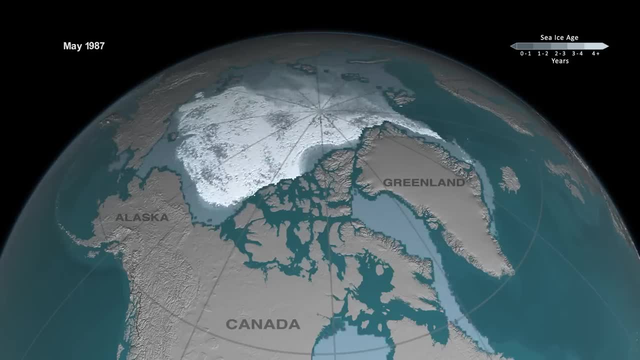 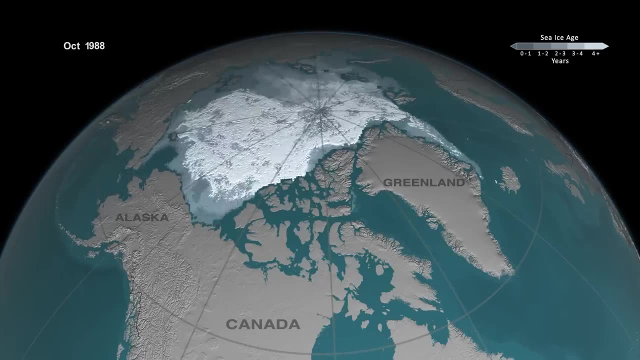 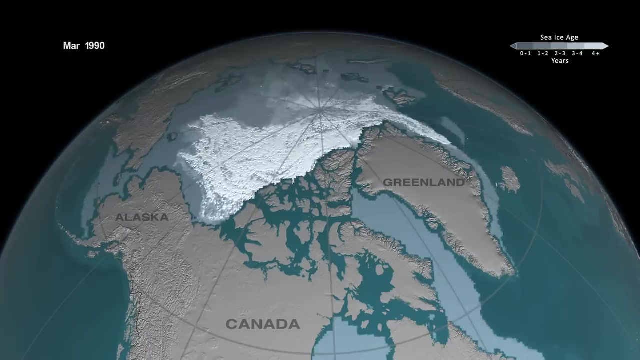 That's the voice of Dr Walt Meyer, senior research scientist at the National Snow and Ice Data Center. What you see in this animation is the ice pulsing out and in with the seasons. In winter, the ice grows out and expands outward. In summer, it contracts inward as 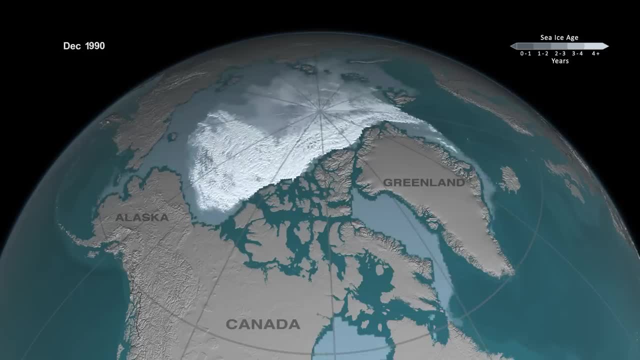 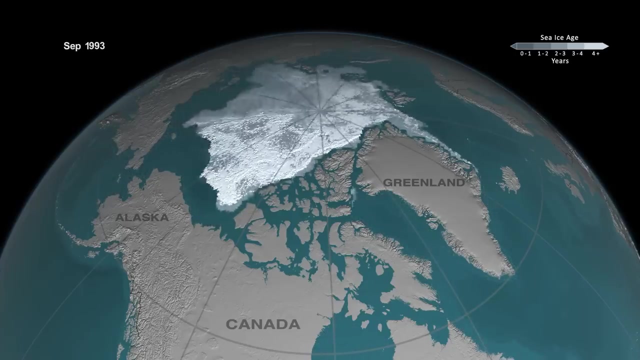 it melts. You see the whiter ice, which is the older ice, moving around the Arctic, being pushed around by winds and currents that move the ice Over the years. the ice pulses around and moves around towards the top along the coast of Greenland. 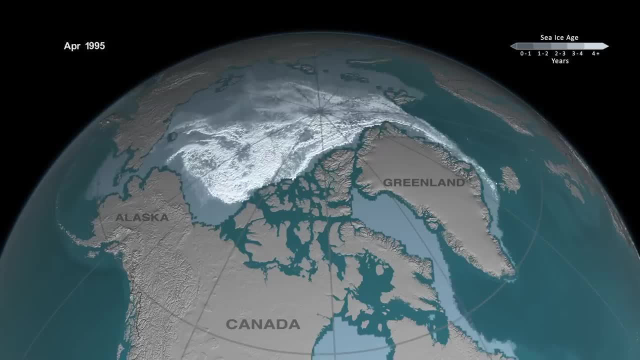 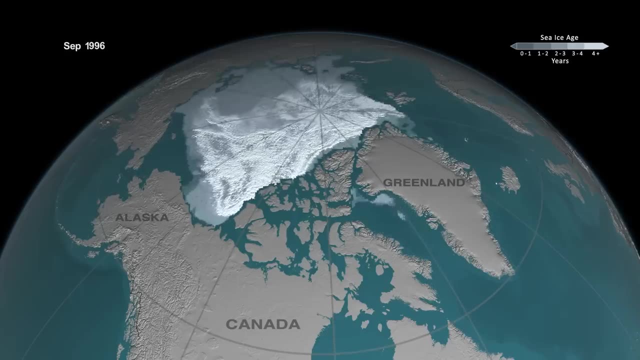 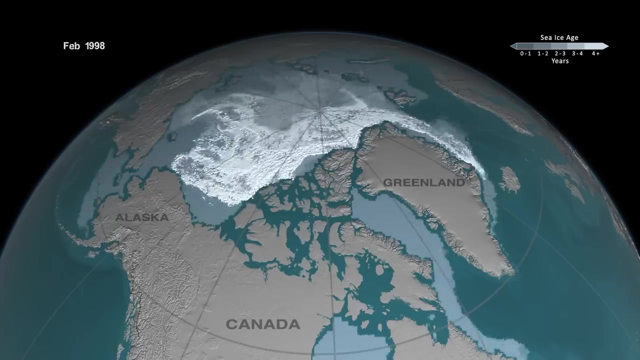 This is the ice age. This is the ice age. The older ice eventually moves out of the Arctic and into the North Atlantic, where it melts. The ice gets replenished within the Arctic because some of the ice survives each summer and grows older, particularly in a region north of Alaska called the Beaufort Sea, where. 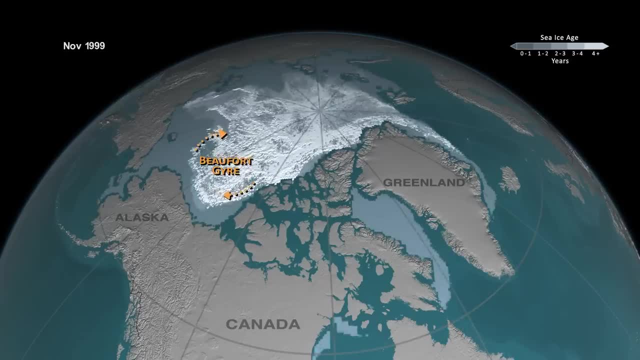 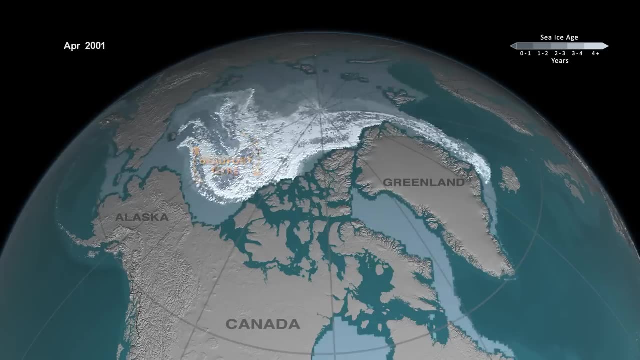 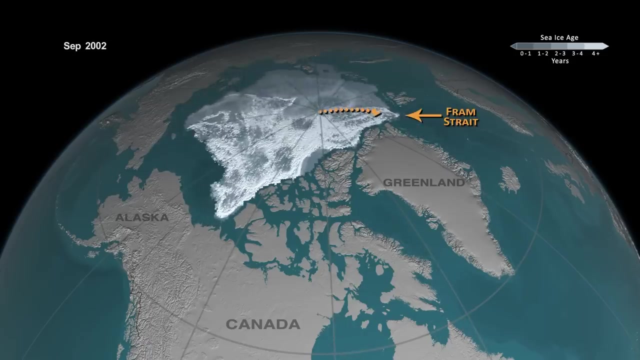 the ice spins around in a clockwise direction called the Beaufort Gyre. That ice can keep spinning around, oftentimes for several years, and gradually getад 2011, getting older and thus getting thicker. Eventually, the ice will spin out of that gyre and go out through Fram Strait.